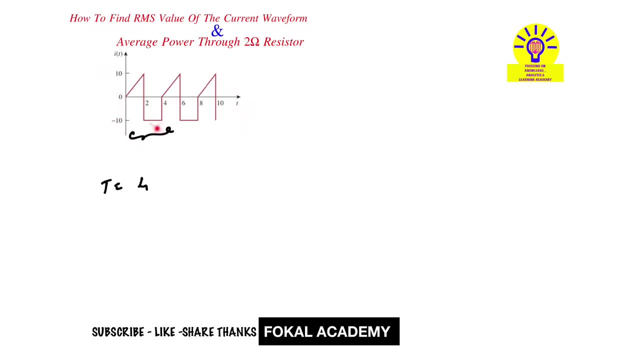 find the wave equation for the given waveform, So then we can easily find the RMS value and average power. So when you observe that: so here 0,, 0 point is there, and here 2,, 10 is there, So then I of t equation is so: 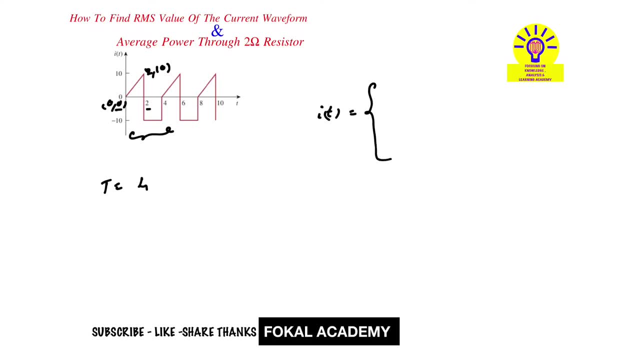 we have two limits are there. So one is 0 to 2, that is 0 less than t less than 2, and 2 less than t less than 4.. So here 2 to 4, the current is constant, that is minus 10.. 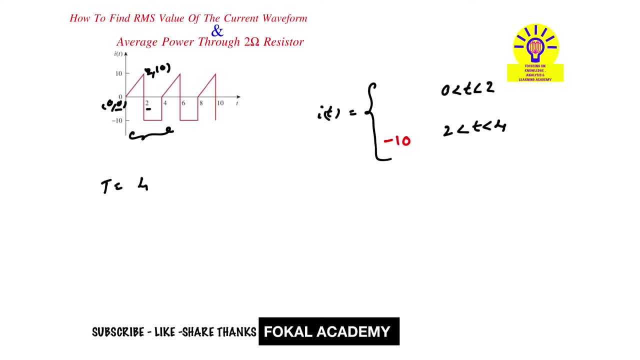 So here minus 10.. Now here we want the equation from 0 to 2, that is, 0, 0 point to 2, 10. So by applying point slope line equation formula we will get line equation, So that 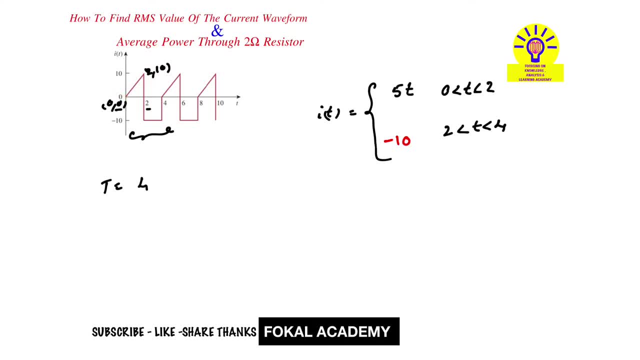 is equal to phi t And this is the current equation for the given waveform. Now we are going to find RMS value. So we know that I RMS equal to 1 by t integral of here. time is from 0 to 4, 0 to 4, I of t whole square dt under root. 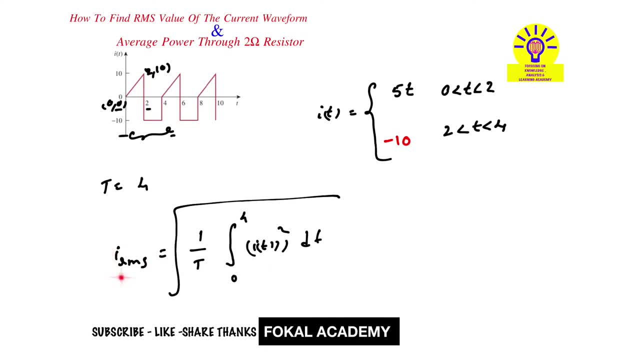 Now, by applying this formula, we will get RMS value for the given waveform. Here t is the time period for the given waveform. we got 4 and here I of t, current waveform. we have two limits. are there? This is a different integral. Now apply two limits, So then it becomes square root of. 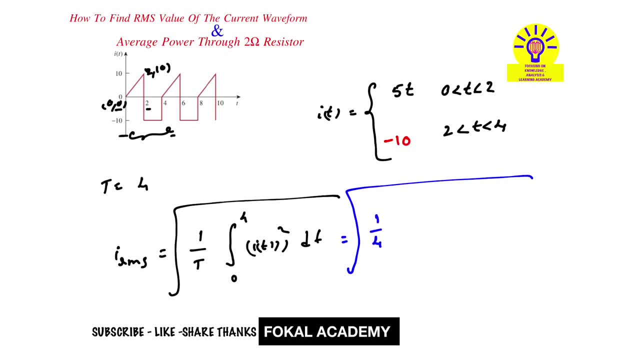 1 by 4, and here the limits are: 2 are there, So it is different integral and convert into two functions. So that is integral of 0 to t one function, another is integral of 2 to 4.. Now here in the limits, this is the limit.